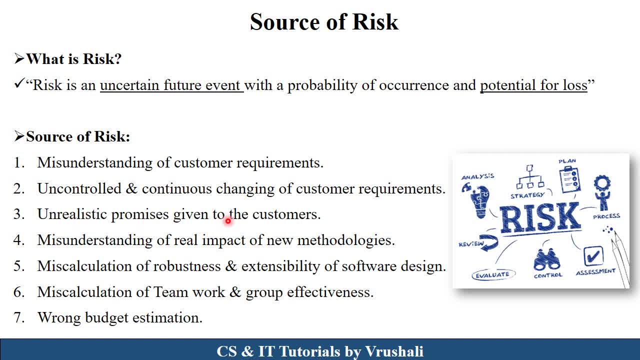 unrealistic promises given to the customer In particular project. there are different but sometimes these modules will not be possible for implementation purpose, but still developer give unrealistic or fake promises to the customer. the next reason is misunderstanding of real impact of new methodology in project. there are different. new methodologies have used but developer didn't know. 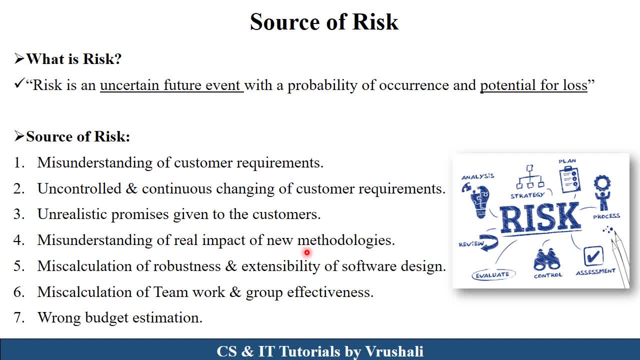 about their usage and about their impact of particular project. the next reasons are miscalculation of software design and software team. sometimes proper software team have not alluded to every software development lifecycle phase or they didn't have some ability and required skills. and the last reason is: 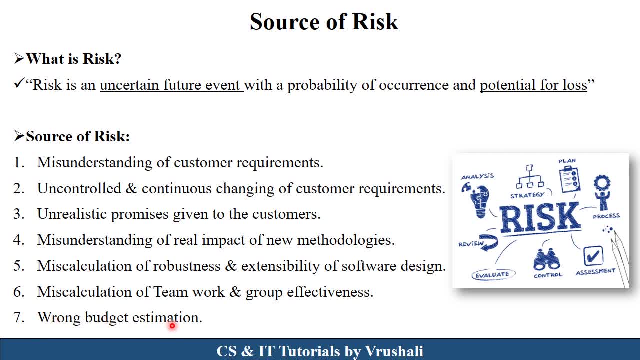 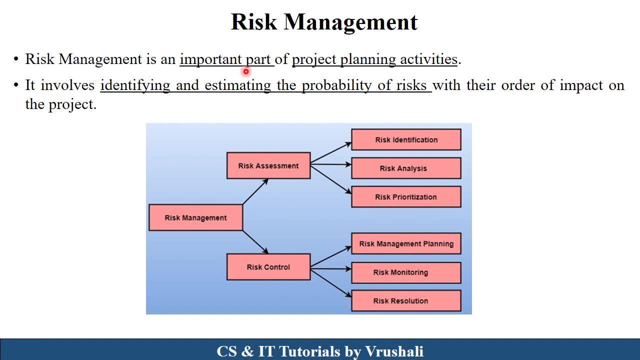 wrong budget estimation. sometimes proper funds have not provided to the particular project. so these are the different reasons. that's where risk will be generated in your project now. the next reason is miscalculation of software design and software team. next topic is risk management. risk management is an important activity in 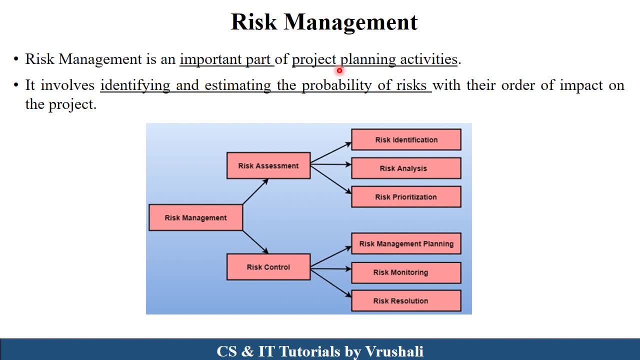 planning phase of software development lifecycle, which is performed by the project manager. see here in this diagram, risk management having two major activity: first, risk assessment and second, risk control. in risk assessment there are total three activity. first, they identify risk, that is risk identification. then analysis of risk, that is risk analysis and risk. 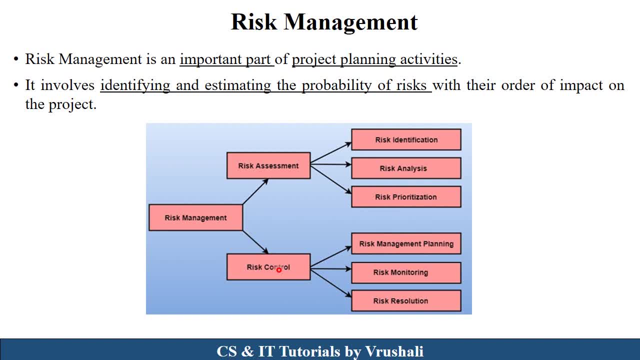 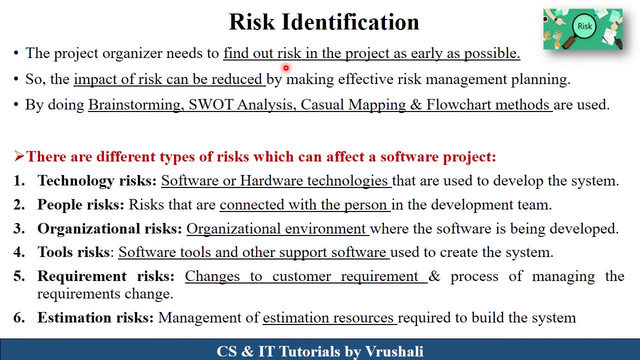 priorities, characterization. and the next one is the risk control. risk control means, after identifying risk, they provide risk management planning, risk monitoring and risk resolution. now let's discuss this risk management process in detail. the first task is risk identification. project manager first identify which type of risk will be generated in future in particular project. this risk identification process perform as early risk function that all criterialies will be didnt as such, risk performance will be an chief priority and its drown the risk off to man's areas problem. alleviate risk and relationship, and the rest two factor values will be the outcomes. financial policy risk management planning providers can conduct. so this is toward. 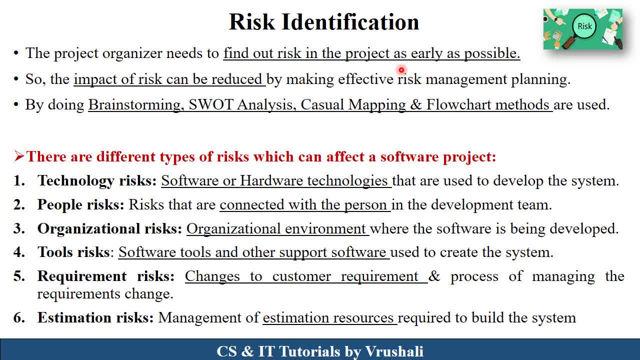 as early stage of development or before start of development. they also identify impact of that risk in particular project. for that purpose they conduct different activities like brainstorming session. project manager arrange group discussion of different stakeholders to discuss which type of risk will be generate than strength, weakness, opportunity and threat. 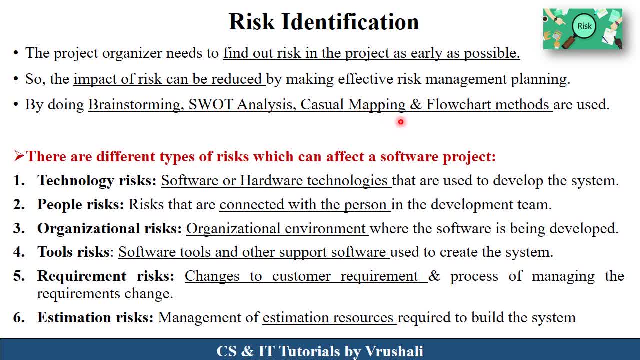 analysis of particular project and after that casual mapping. and flowchart methods means: first they mention some rough design of particular project or rough prototype of particular project and by analysis of all those things they decide which type of risk will be generate. now there are different types of risk which affects on software project. the first one: 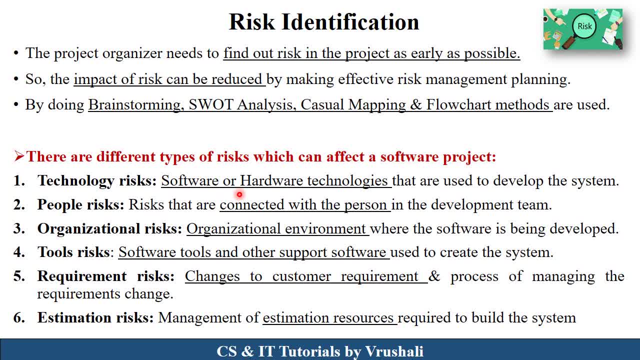 is a technology risk in particular project. there are different software and hardware technologies have used, but sometime this software and hardware technologies have used, but sometime this software and hardware technologies are not suitable on particular platform or particular operating system, or sometimes it get delay while purchasing a particular software and hardware at that time. 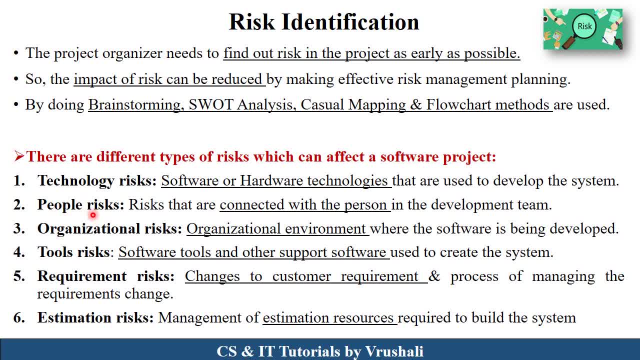 technology risk will be generated. the next risk is a people risk. sometimes there is no communication between all the software development team or they required some less abilities and skills regarding particular project. then people risk will be generated. the next one is a organizational risk. sometime organizational environment is not suitable for particular project, then organizational risk. 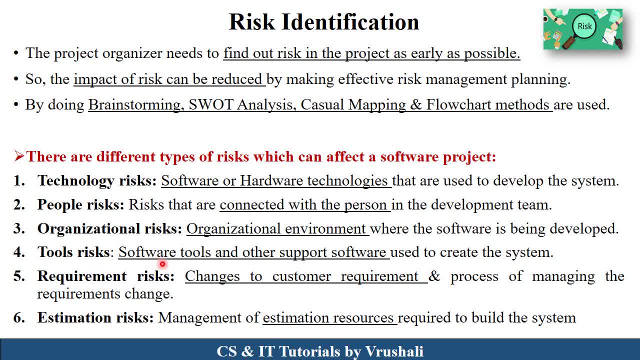 will be generated tools risk in particular project. there are different software tools and other soft support softwares have used, but sometimes these tools are new or updated, so at that time tools risk will be generated. the next one is a requirement risk. sometimes customer requirements are continuously changing, so at that time requirement risk will be generated, which is very impossible. 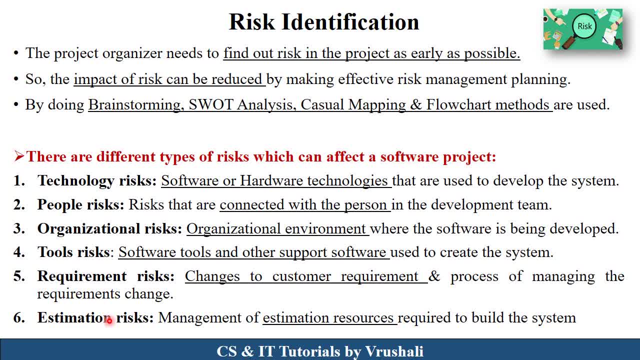 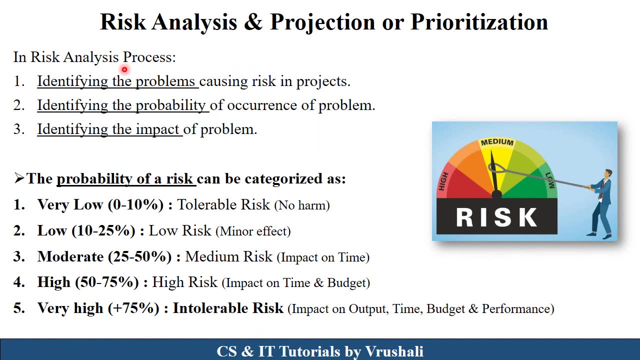 for maintaining all the requirements. and the last one is a estimation risk. sometime proper schedule and proper cost have not provided to the particular project, at that time estimation risk will be generated. so these are the different types of risk will be generated in particular software project. now the next is risk analysis and projection. so after identifying risk, the next step is risk. 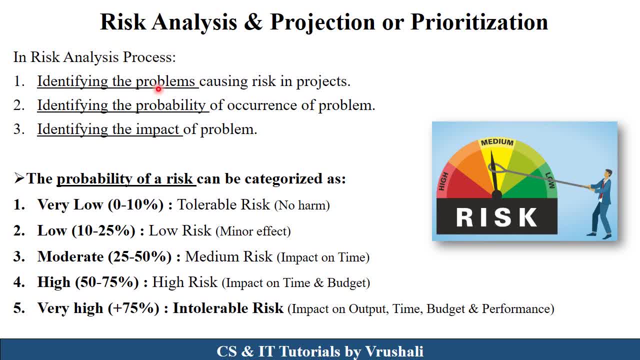 analysis here. these are the process: first day of the project. the next day of the project. the next day of the project they identify problems which causes a risk in particular project. after that they identify probability of risk. see here: suppose a particular risk is tolerable. risk means they provide no harm. 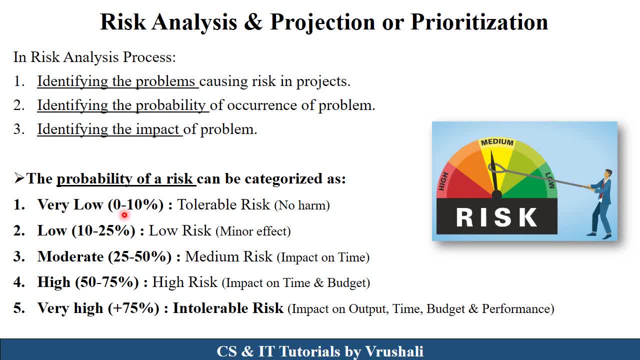 to the particular project. so that is very low risk. that is 0 to 10 percent. some risks are minor effect on particular project. that is low risk which under 10 to 25 percent probability. the sum rest is medium rest. sometimes your product will get delay or your project will get delay, as per the 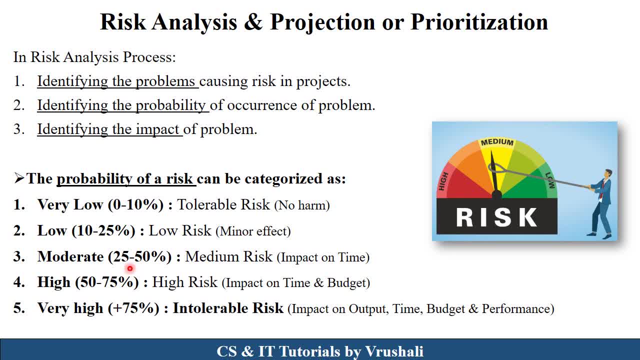 customer requirement. so at that time moderate risk will be generated. sometime your project will get delay and they didn't have a proper budget. then high risk will be generated and sometimes your project output is not as per the customer requirements. their delay in time, their loss in particular budget and there is a low performance is there. so that is intolerable. 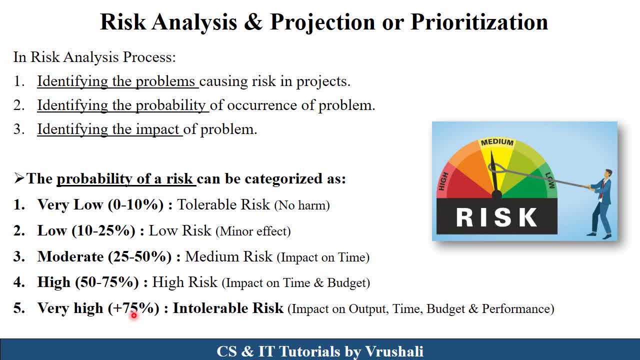 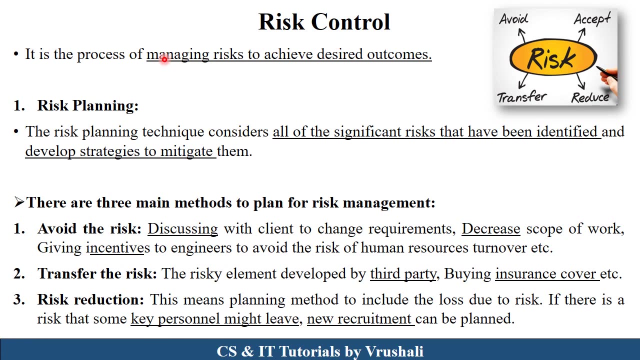 risk, which is very high, means more than 75 percent probability. so this is a probability of risk. this is called as risk projection or prioritization. so after analysis they identify probability of risk and according to that they provide the solution. now the next one is a risk control. basically, risk control means to manage all the risk that have. 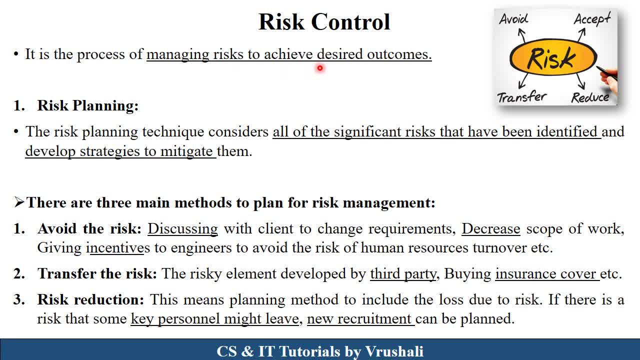 generated in particular project which achieve a particular design outcomes. the first method is risk planning. project manager plan all the strategy and all the techniques to minimize risk in particular project. there are total three methods in risk planning. first, avoid the risk. for that purpose, project manager discuss with client. 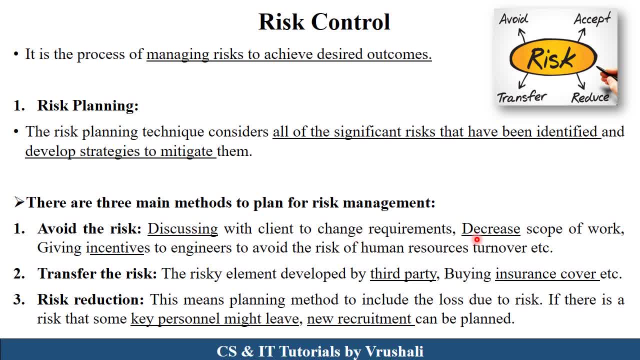 about their changing requirements. then they also discuss the final aim of your particular project. also they giving some insensitive to engineers. they decide proper human resources as per their abilities and skill to the required particular project. in this way they avoid risk in particular project. next one is a transfer. the risk see in particular project there. 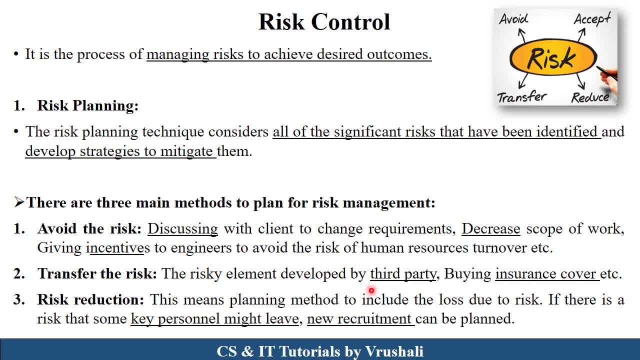 are different models, but some modules they transfer to the third party for development purpose as per their skills or as per their requirements. that is, transfer the risk. and the last one is a risk reduction. see in particular project. there is a plan a for development, but project manager decide plan b and plan c. also, if plan a didn't work then they move to plan b. so there, 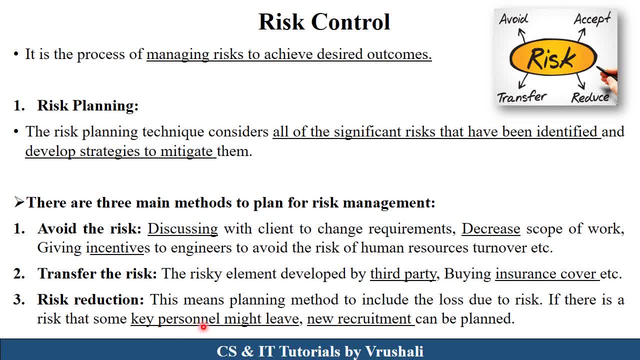 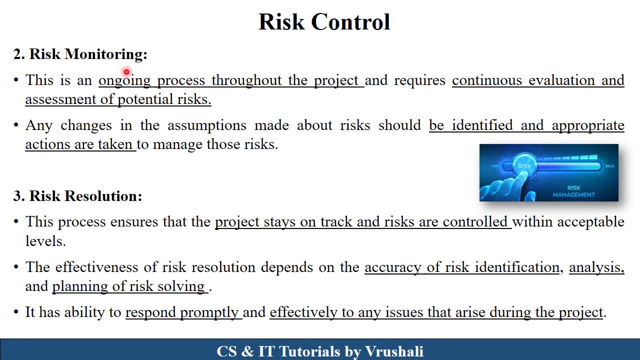 is a risk reduction in that suppose a key personal means, suppose project manager leave a particular project, so new recruitment as per the skill of project will be planned. this is called as risk reduction. now the next method is risk monitoring. so risk monitoring basically means they monitor ongoing complete process of software development process. 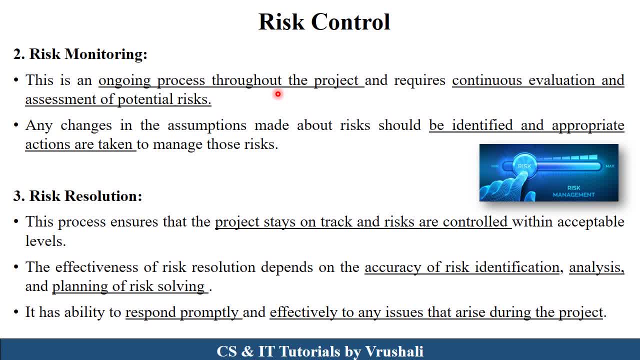 life cycle. they monitor requirement gathering phase, design phase, development phase, testing phase and, after that, deployment phase. they monitor all these phases and to check that, whereas any risk, problems or issues have occurred in particular project or not, and if particular risks have occurred, they provide some appropriate actions or strategy. 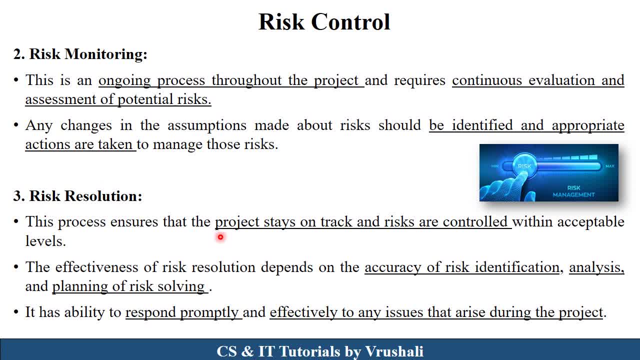 the next method is risk resolution. so basically, risk resolution means they stay track on particular project, they see specific problem, as i told, they canract on others cost, they get to know đa tool or They find out the efficiency of accuracy of risk identification means how project manager 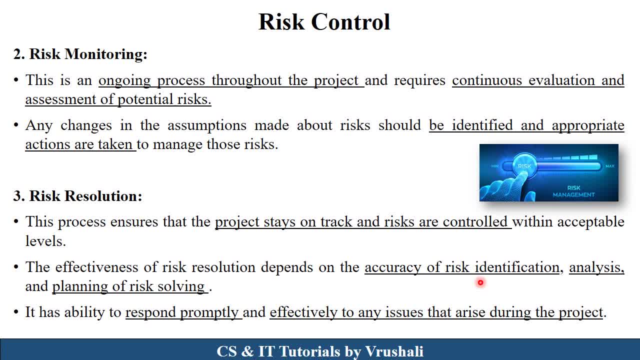 identified risk accurately in particular project, how project manager analyze all the risk and how project manager provides strategy or development plan to solve those risks. So to monitor or to calculate all the effectiveness are called as risk resolution. So these are the risk control methods. 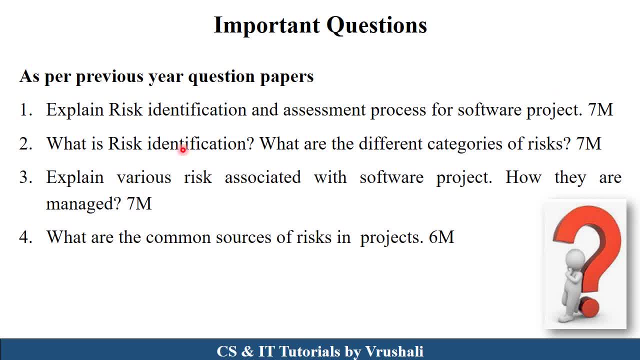 Now, as per your previous year question paper, these questions are most important, like: explain risk identification and assessment process of software project, for 7 marks. Then what is risk identification? different categories of risk- for 7 marks. Then. explain various risks associated with software project and how they are managed. 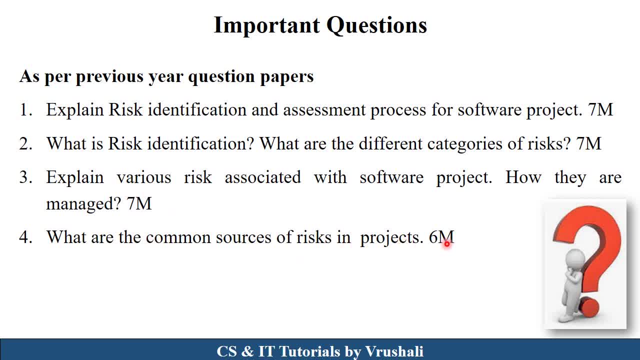 for 7 marks and what are the common source of risk in particular project for 6 marks. So you have to prepare this topic completely. In next session we will discuss about RMM- plan for solving RMM- Solving all the risk management issues.